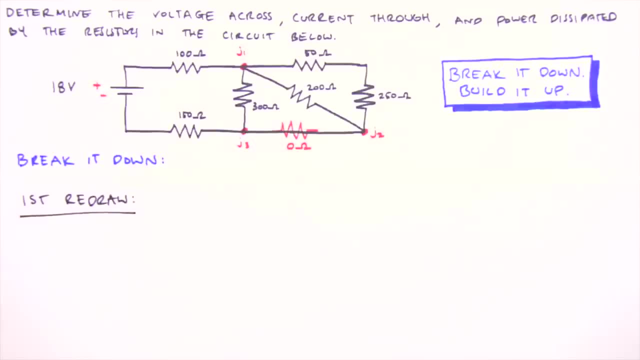 current path, clockwise from positive to negative into a unidirectional one left to right. I find it useful to imagine grabbing the positive side of the battery with your left hand and the negative side with your right, then breaking the battery apart and stretching the circuit out onto. 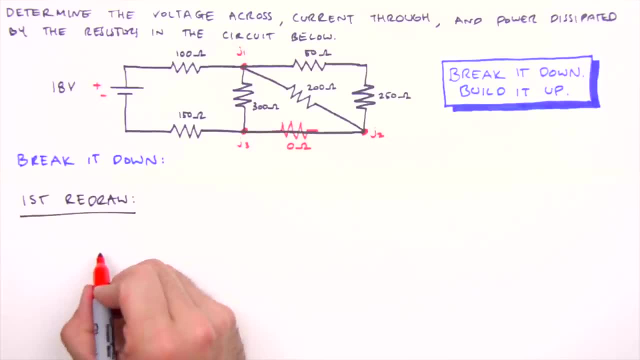 the page below. So we put the positive side of the battery here on the left and translate the rest of the circuit After leaving the positive side of the battery. the current encounters: the 100 Ohm resistor first, so we'll write that here, And thereafter the current encounters, junction one. 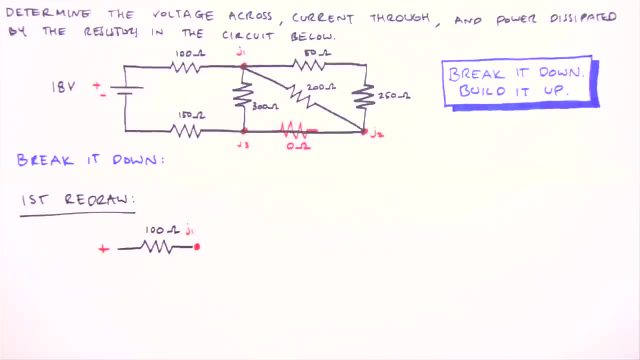 There's a three-way split at junction one, which means these legs are in parallel. So we'll draw them geometrically parallel below. So this top leg has a 50 Ohm resistor and a 250 Ohm resistor follows it, so they're in series And the top leg terminates right here. 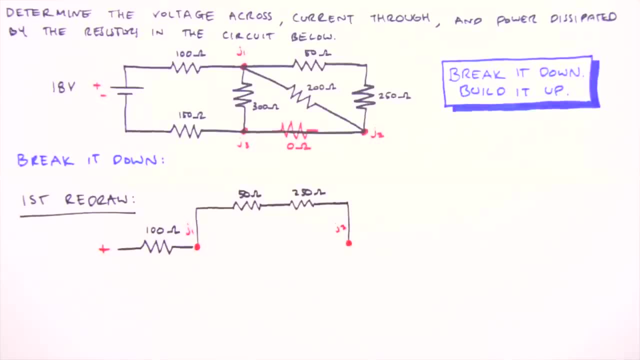 at junction two. There's another leg that begins at junction one and terminates at junction two, and it comprises this devilish diagonal resistor. Despite its menacing appearance, it's just connected in parallel with the top leg, so we'll draw it simply, spanning the gap between. 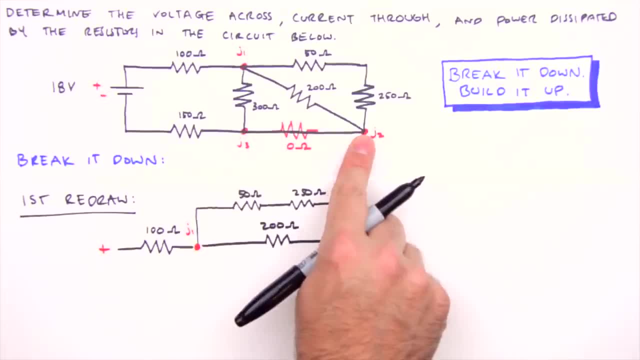 the two junctions below. After junction two we have this bottom leg with our zero Ohm resistor. We'll put that to the right of junction two here And then we get to junction three. Between junction one and junction three is a single 300 Ohm resistor, so it is in parallel with. 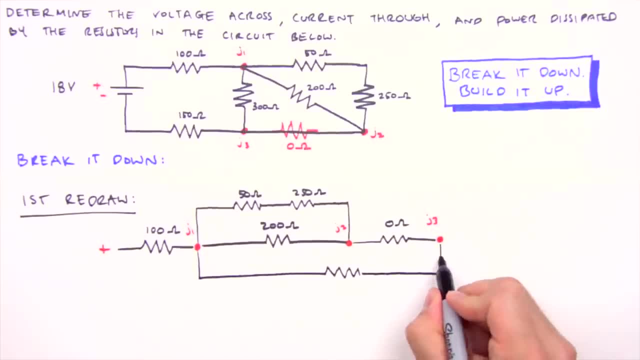 the four previously drawn resistors. We'll depict this by dangling one long leg from junction one and junction three. Finally, following junction three, we have a single 150 Ohm resistor, leading us home to the negative side of the battery. So we draw the 150 Ohm resistor here. 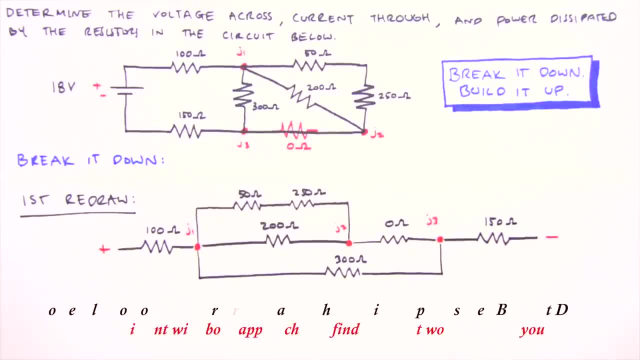 and finish with the negative side of the battery on the right. And that, my friends, is our first redraw. You can see what I meant by breaking the circuit apart and stretching it onto the page. Now we can easily determine our first equivalent resistance. We'll start with. 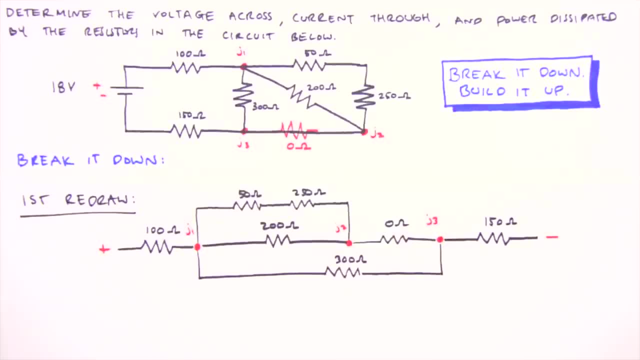 the resistors that are furthest from the battery and determine their equivalent resistance. So, starting inward from the positive and negative sides, we find that the 50 and 250 Ohm resistors fit the bill. If you're ever unsure where to start, resistors in series are always a good bet. 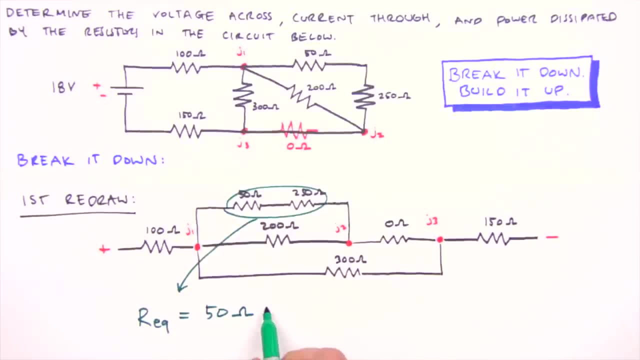 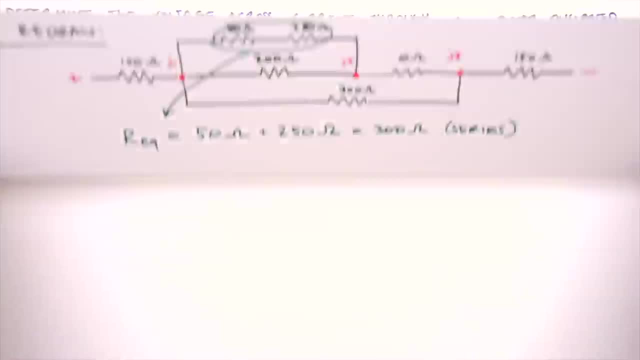 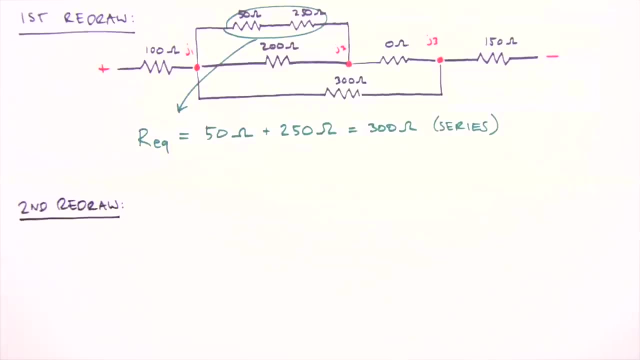 So the equivalent resistance for these two resistors is 50 Ohms plus 250 Ohms, which equals 300 Ohms. This is how we calculate equivalent resistance for resistors in series: simply sum their individual resistances And this brings us to our second redraw. We'll redraw the. 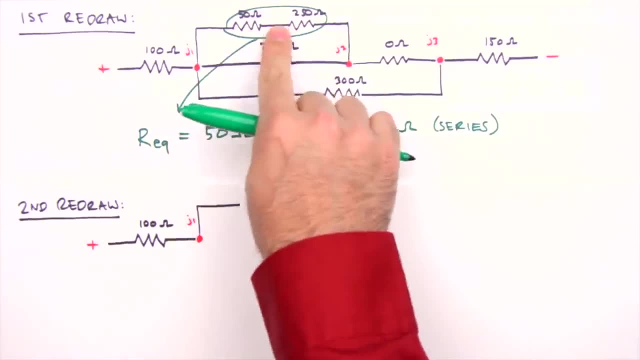 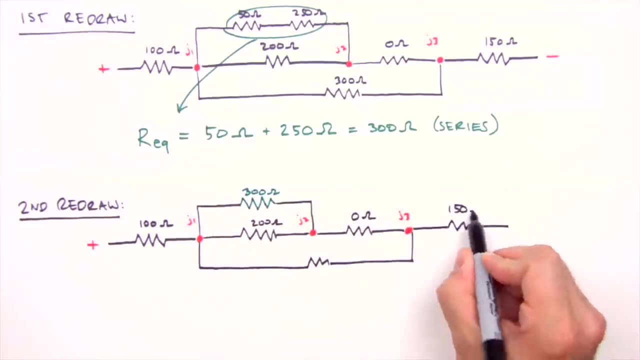 circuit, but in place of the 50 Ohm and 250 Ohm resistors we'll draw a 300 Ohm resistor. like so: Once we finish our second redraw, we again turn our attention to the circuit diagram and determine. 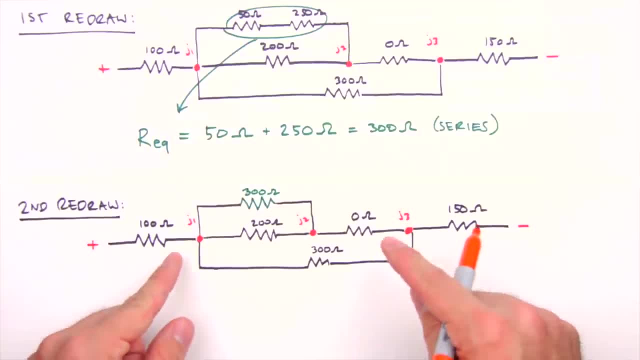 the resistors furthest from the battery. Moving inward from the sides of the battery, we find that these two resistors are the next to be combined. We calculate their equivalent resistance differently because they're not in series but in parallel with one another. So for our 300 and 200 Ohm resistors, 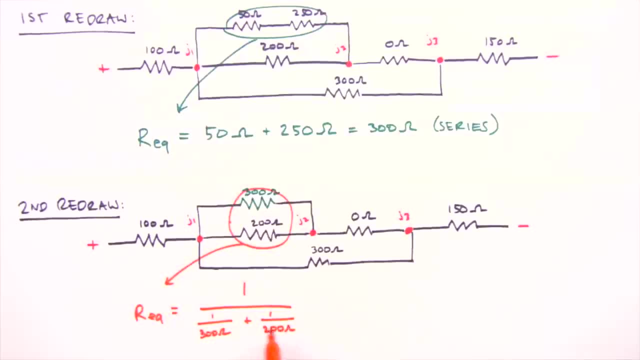 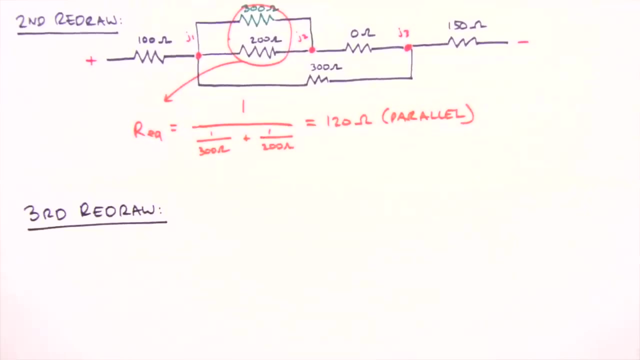 we'll divide that by 1 over 300 Ohms plus 1 over 200 Ohms, which equals 120 Ohms. So for resistors in parallel, the equivalent resistance is equal to the reciprocal of the sum of the reciprocals. Okay, moving on to our third redraw. Here we'll have the same circuit. 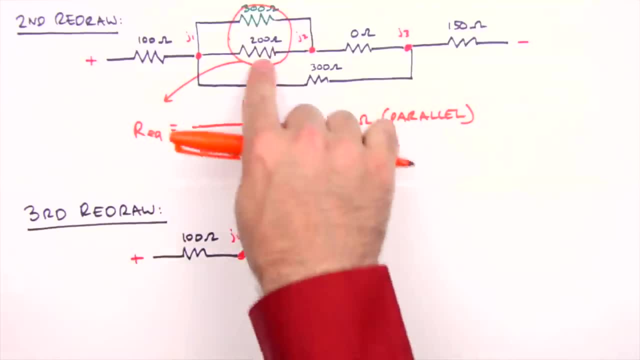 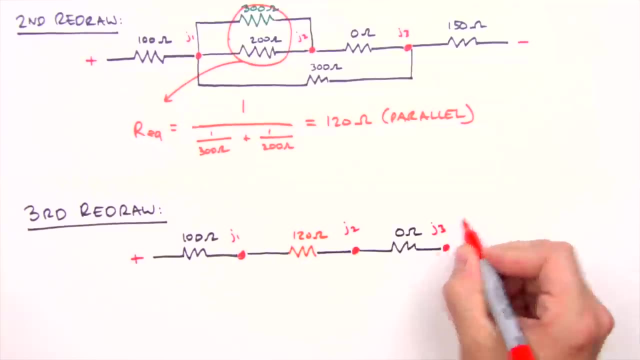 as depicted in the second redraw, except that we replace the 300 and 200 Ohm resistors with their resistive equivalent, a single 120 Ohm resistor. Starting to get the hang of this? If not, don't panic, we've got a couple more redraws with which to practice before we're done breaking it. 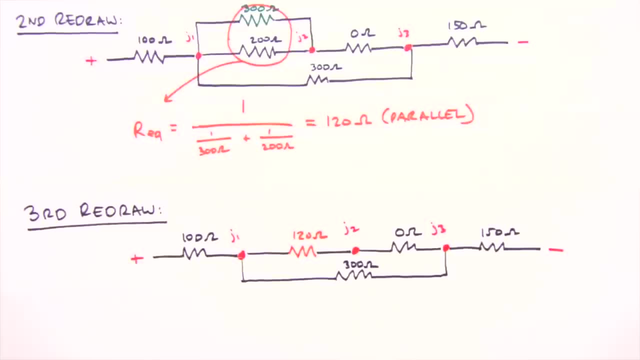 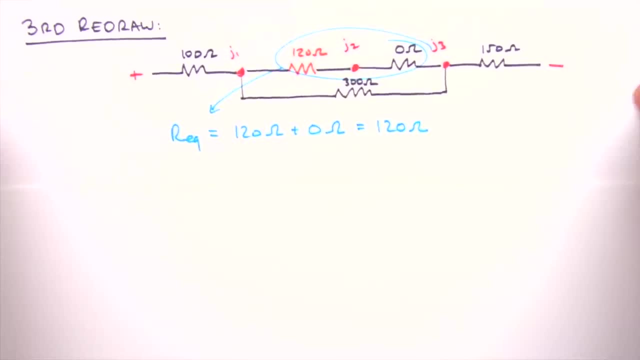 down. So which resistors are next? You guessed it: the two that are in series. So we just add their resistances together. Not a very exciting equivalent resistance, I admit. but note that junction 2 will not be present in our fourth redraw, So we wash, rinse, repeat. replacing: 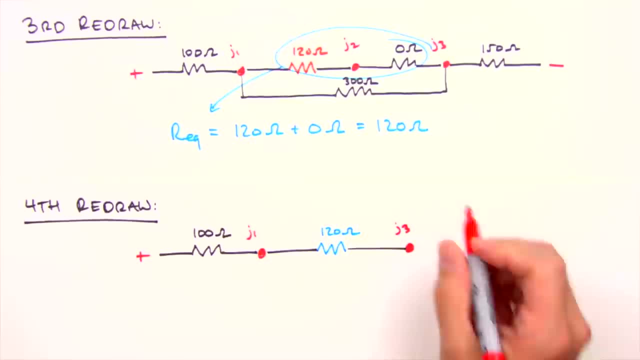 these two resistors with their resistive equivalent, and perhaps by now you've identified the next resistors to be combined, The two in parallel, right here. So for their equivalent resistance we'll have 1 over 1, over 120 Ohms. 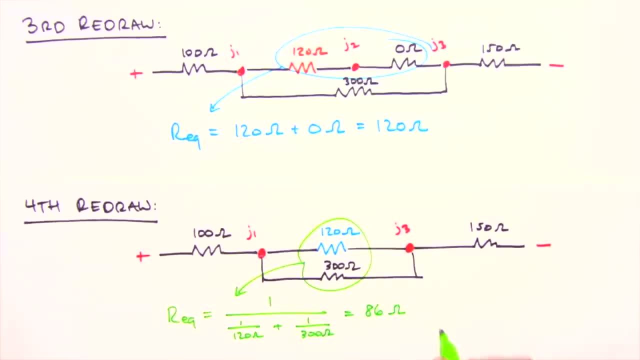 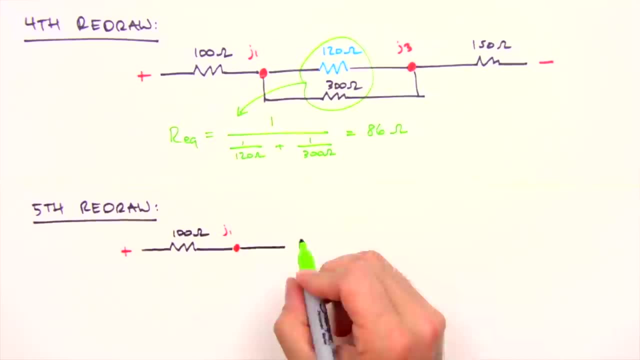 plus 1 over 300 Ohms, which yields 86 Ohms. Again, we redraw the circuit, this time replacing the two parallel resistors between junction 1 and junction 3 with our 86 Ohm resistor. This redraw leaves us. 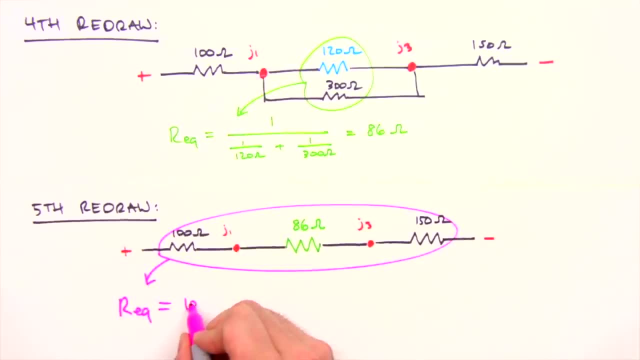 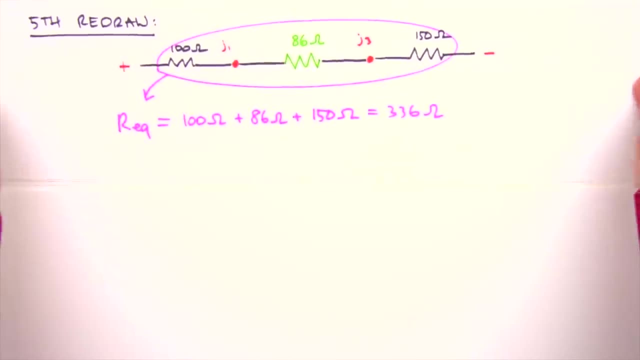 with three resistors to combine. They're in series, so we just sum their resistances, which yields an equivalent resistance of 336 Ohms, Which brings us to our final redraw. We've reduced our initial six resistors to a single equivalent resistance, which means we're done breaking it down If we 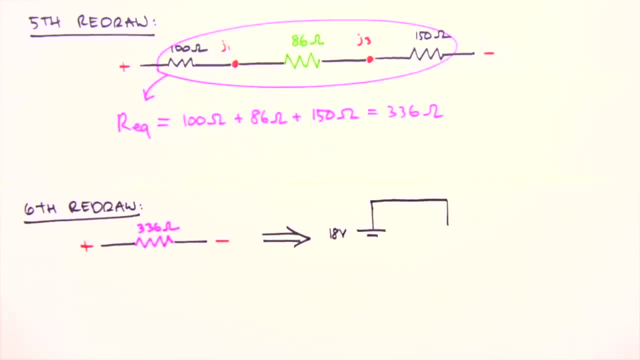 bend our circuit back together, reconnecting the positive and negative sides of the battery, it should be clear that we're left with our old Ohmic friend, the simple circuit, And, as far as the battery is concerned, that's all there ever was, No matter the circuit's configuration. 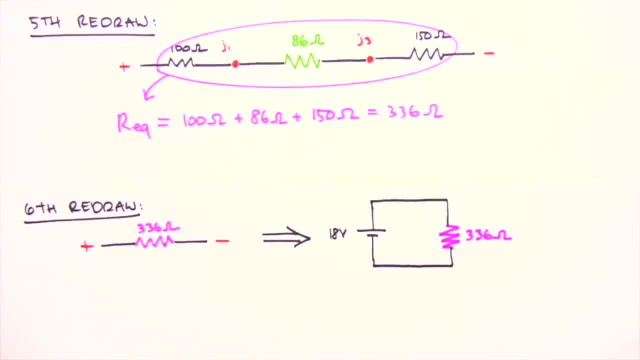 the battery only sees an equivalent resistance and supplies the circuit with a corresponding current. How the circuit divvies up this current depends on the configuration, So we'll label the current leaving and re-entering the battery as I0.. See, I told you we'd come back to drawing our 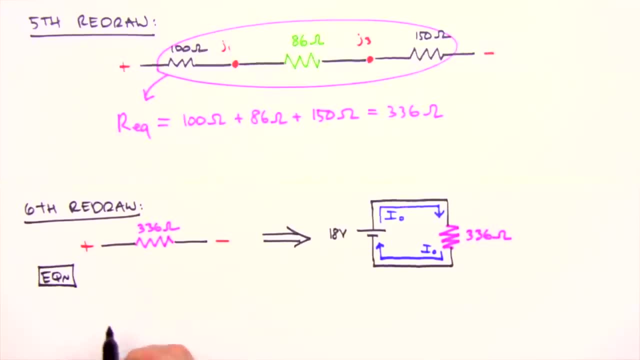 currents. And now we'll determine a value for I0 using Ohm's law. We write: V equals I, R, which will solve for I, which, in this situation, gives us I0 equals the source voltage divided by the equivalent resistance. Inserting our values, we find that I0 equals 54 milliamps. Eureka A value. 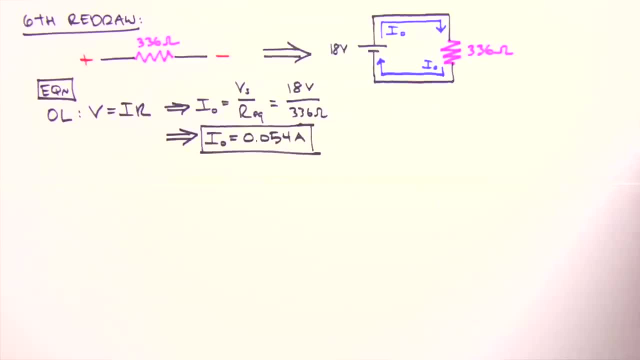 for current leaving and re-entering the battery marks the halfway point in our analysis, which means it's time to build it up now. To build our circuit back up to its original configuration, we'll move through our series of redraws in retrograde. 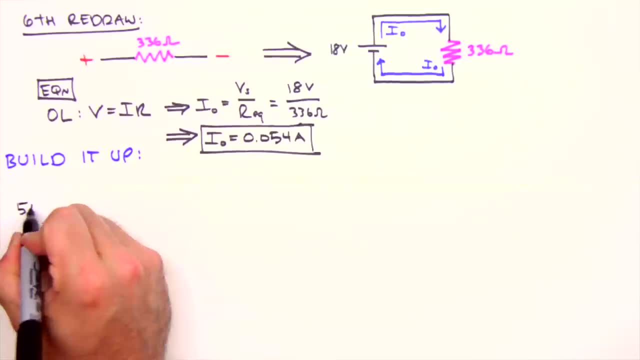 Determining the values for voltage across and current through each resistor. as we go, So we begin building it up by revisiting our fifth redraw. By the way, I'm redrawing my redraws here for the sake of neatness, but to save on time and paper at home. 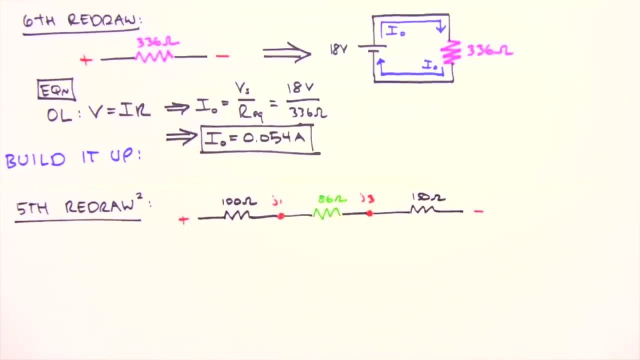 just simply mark up your old redraws. Okay, we know that I0 passes through the resistor representing the equivalent resistance of these three resistors And since there's only one path for the current, we know that I0 must pass through each of the three resistors. In other words, series resistors experience the same current. 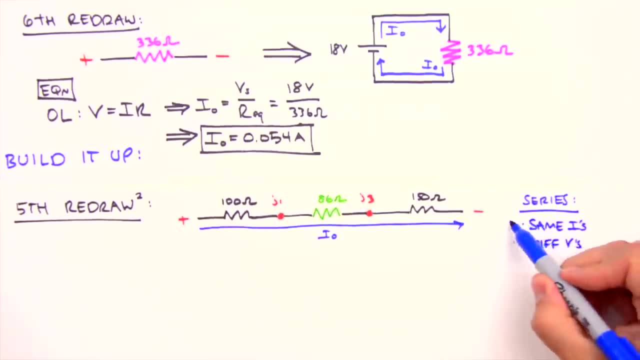 but provided their resistance values differ, they experience different voltages. Knowing the current through the resistors, we can now determine the voltage across them using Ohm's law. So for the 100 ohm resistor, we apply Ohm's law and we get the voltage across the 100 ohm. 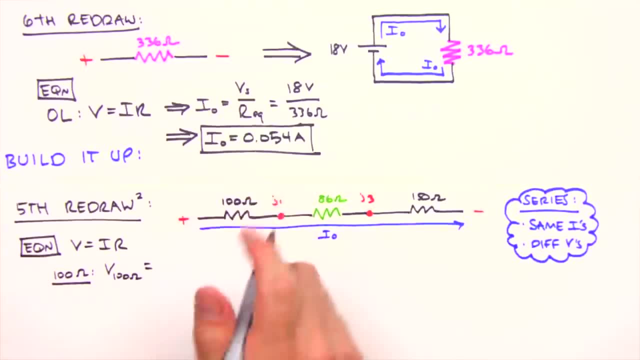 resistor equals the current through the resistor, which is I0,, that's 0.054 amperes times the resistance of the resistor, Which is, of course, 100 ohms. This yields a voltage drop across the resistor of 5.4 volts. 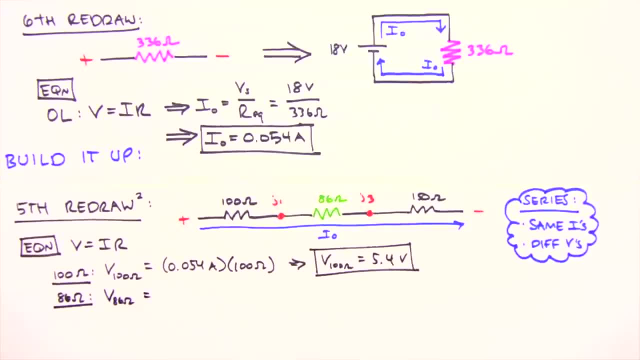 Now for the 86 ohm resistor, V equals I, that's 0.054 amps times R, 86 ohms, which equals 4.6 volts, And for the 150 ohm resistor, 0.054 amps times 150 ohms, which equals 8.1 volts. 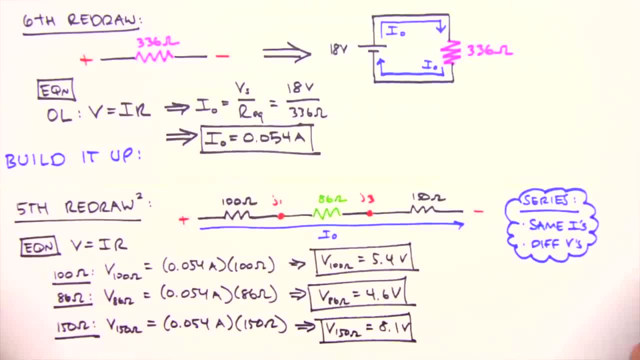 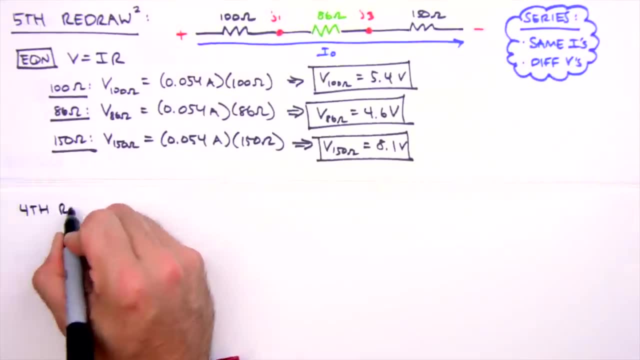 Now, at this point we could determine the power dissipation, but we'll just wait to calculate power until the end of the problem, when we tabulate our solutions. Next we revisit our fourth redraw, where in junctions 1 and 3 are actual circuit junctions. 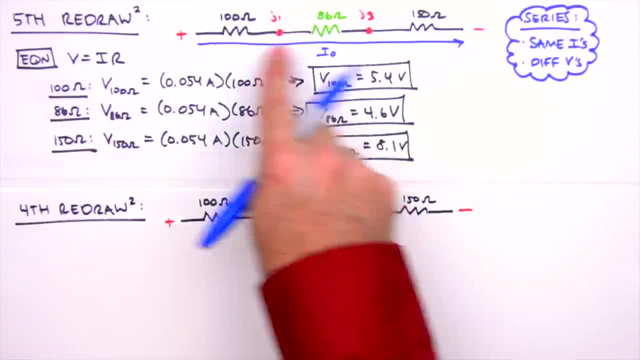 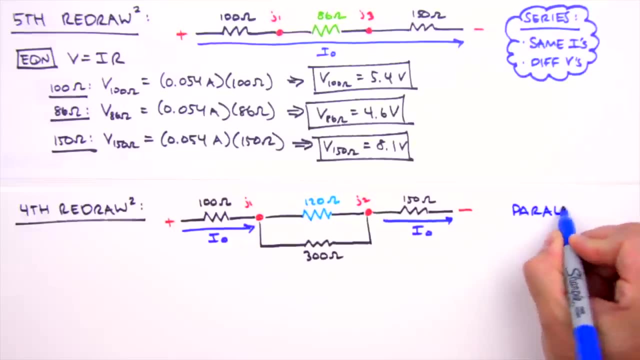 where three or more paths come together. Here we have I0 splitting up into two currents at junction 1.. What do we know about resistors in parallel? Well, we know they'll have the same voltage, but so long as they have differing resistances, they'll have different currents. 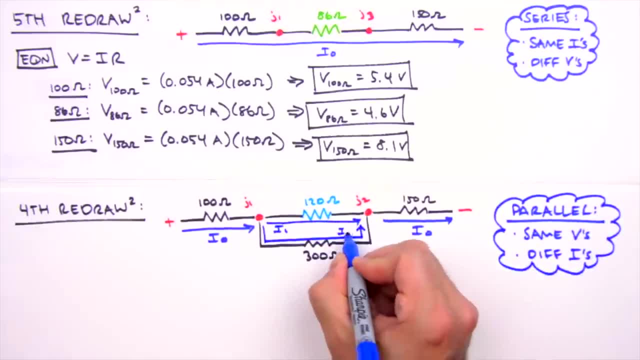 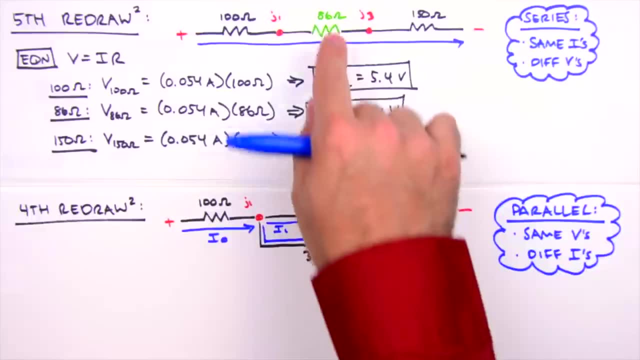 And so we'll label the currents here I1 and I2.. To determine values for I1 and I2, we'll use Ohm's law, but first we need voltages for these two resistors. We know that the voltage drop across the 86 ohm resistor is 4.6 volts, and 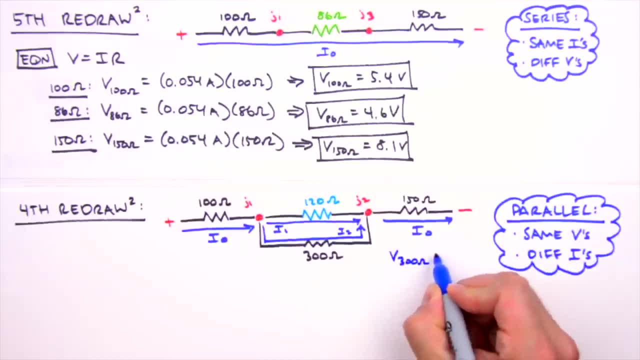 since it represents parallel resistors. that means the voltage drop across each resistor is the same 4.6 volts, And we'll box up this result to save for our solutions. table Solving Ohm's law for current. we determine that the current through the 120 ohm resistor, that is to say I1, equals 0.038. 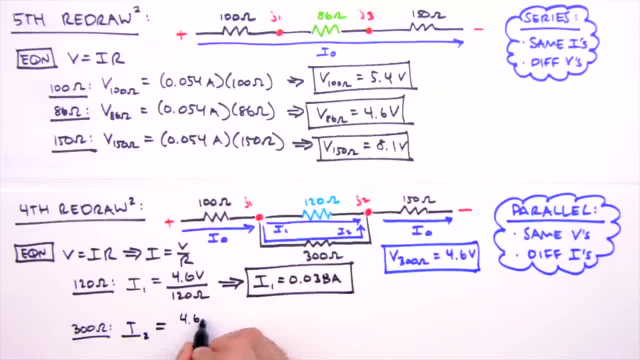 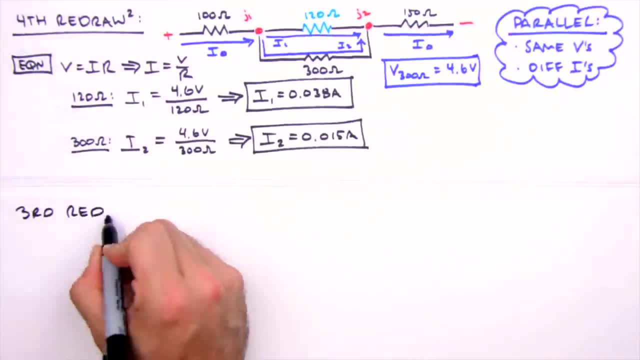 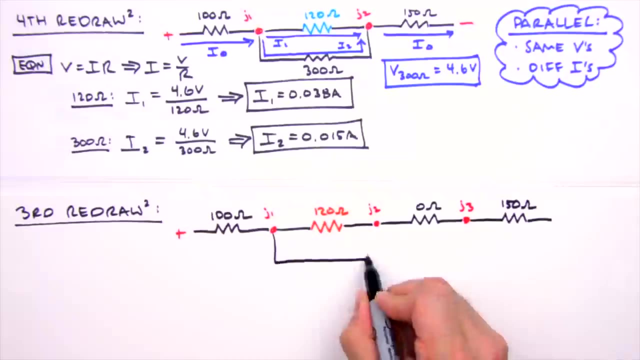 amps. Similar calculation for the 300 ohm resistor yields a value of 0.015 amps for I2.. Now to our third redraw. Here the 120 ohm resistor expands in a rather unexciting way. Out pops a goose egg resistor. I0 doesn't change. I1 passes through both the 120 ohm and 0 ohm resistor. 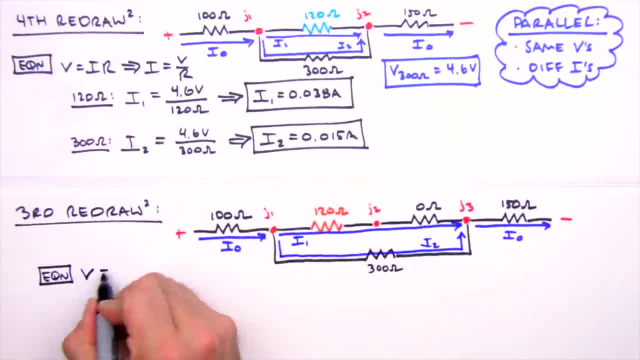 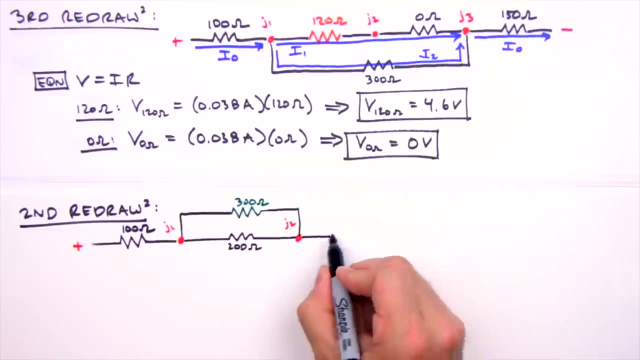 And I2 is the same. We'll run the calculations for the sake of posterity, with the unsurprising result that the voltage drop over the 0 ohm resistor is 0 volts Onward, and upward Or backward depending on how you look at this method. In our second redraw we have an additional leg of 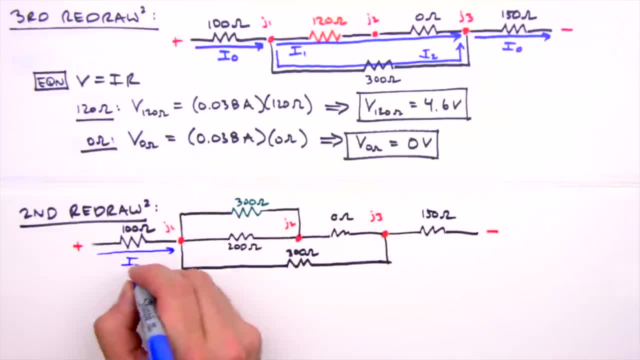 this circuit, which means we need additional currents Again. I0 and I2 don't change, but I1 is now divided between the 300 ohm and 200 ohm resistors here, So we'll call this one I3. 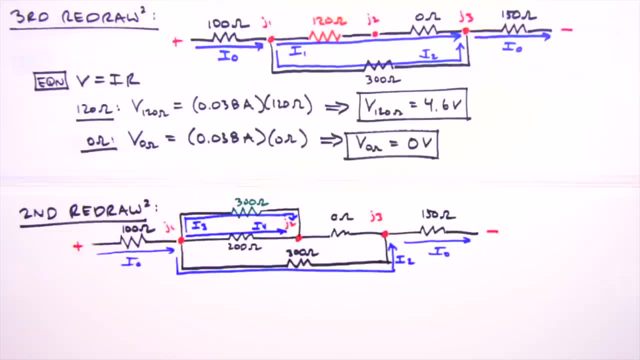 And this one I4.. To get values for I3 and I4, we'll use- you guessed it- Ohm's law. We need voltages first. but because they're in parallel, they have identical voltages to the resistor representing their equivalent resistance. That's 4.6 volts. We'll box that up for the 200 ohm resistor. 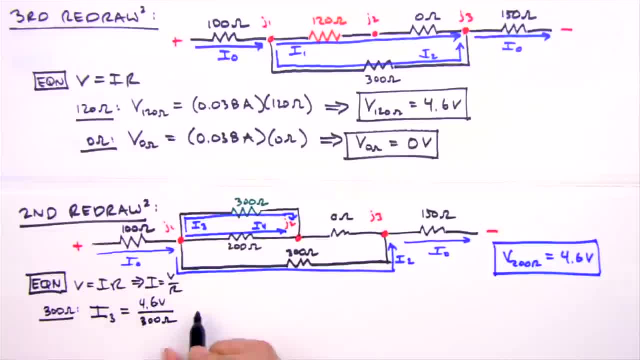 And we determine current values using this voltage. So I3 is 0.015 amps and I4 is 0.023 amps. Got the hang of this. It's 1.05 volts calculated in again. Good, now back to our first redraw…. By the way, you'll likely be studying circuits with 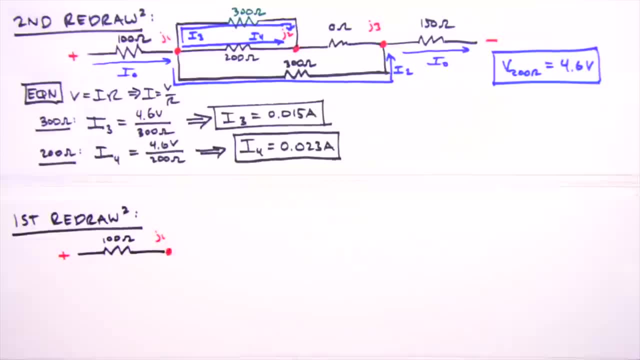 multiple power sources. soon and when you do, you'll need another circuit analysis tool, namely Kirchhoff's Rules. Subscribe to my channel now, and when you need help with Kirchhoff's, come on back. OK, I zero hasn't changed, so we'll draw that one first, The current through this top leg. 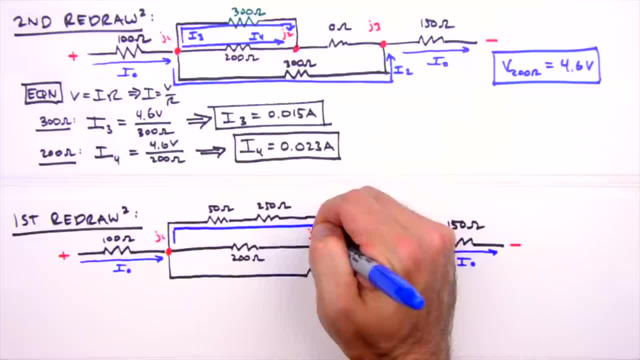 containing the 50 ohm and 250 ohm resistors. That's I3 here, And the 200 ohm resistor. It's connected to I4.. 1. team the current through the bottom leg, that's I2,. 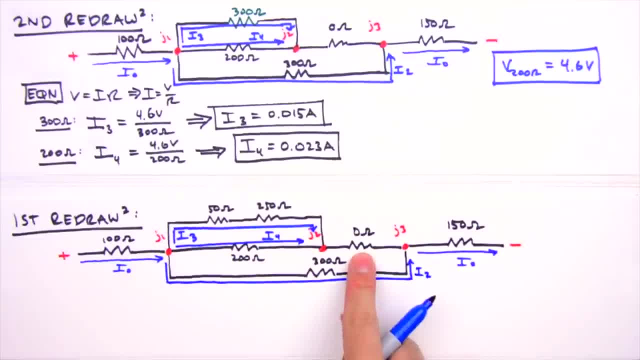 and it looks like we forgot to label the current through the dummy resistor in our last redraw. That's just I1.. So the final pieces of our circuit puzzle are the voltages across the 50 ohm and 250 ohm resistors.